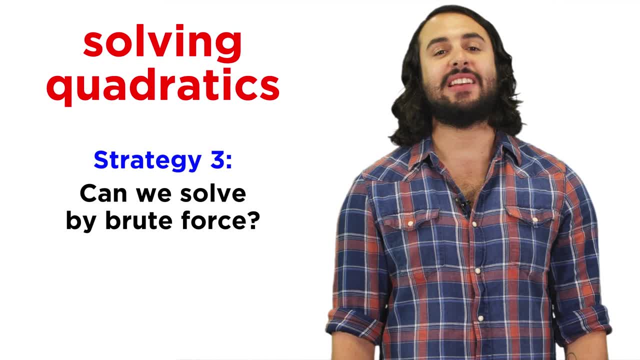 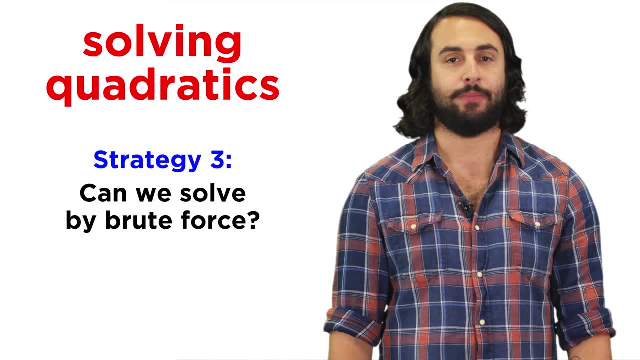 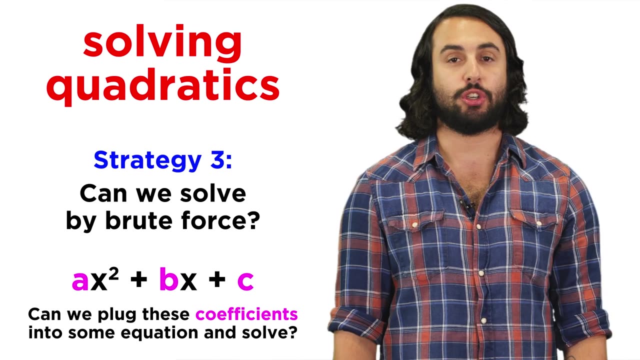 possible to perform. In general, it would be nice to have another method where we can solve by brute force rather than having to perform some algorithm. We need an equation where we can simply plug in the coefficients of the expression and get the solution. Fortunately, there is such an equation. 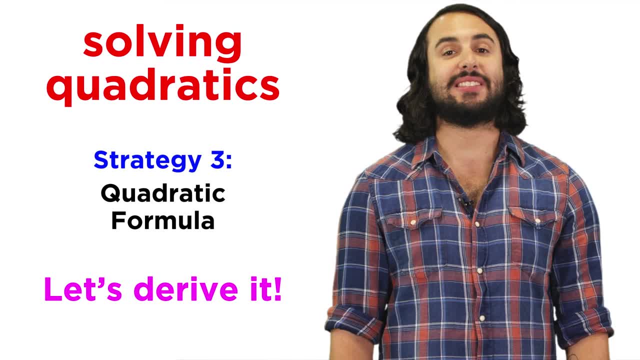 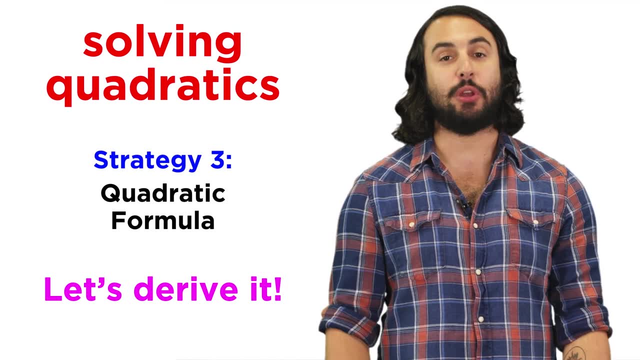 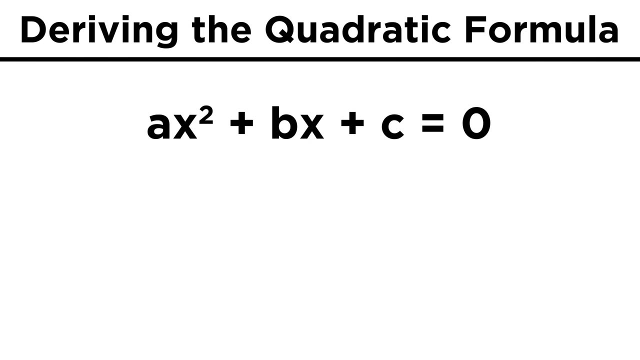 It's called the quadratic formula. But instead of simply looking at it, let's derive the equation, as derivations always help us appreciate the beauty of math that much more. Let's start with a general polynomial equation: ax squared plus bx plus c equals zero, where 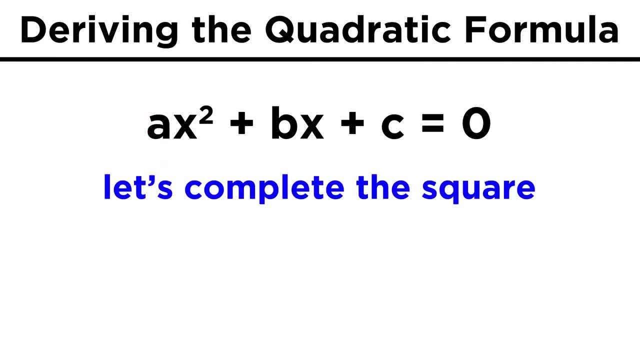 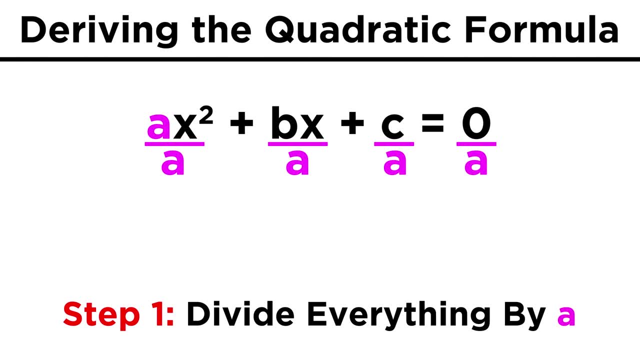 a is not equal to zero. Let's try to complete the square just as we learned before, but with this general form instead of a specific example. Remember the first thing we would do is divide everything by a, because it's easier if 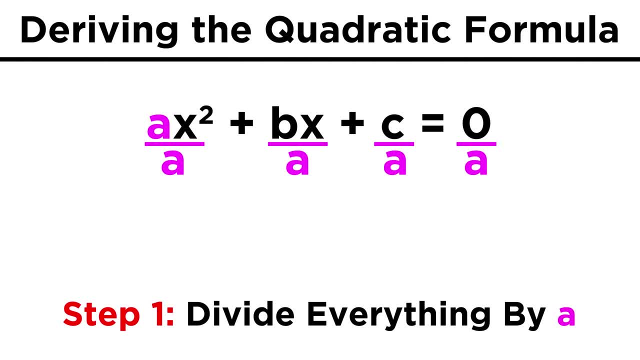 there is no coefficient operating on the x squared term. That means we get x squared plus b over a times x plus c over a equals zero. Then, as usual, we bring the last term to the other side of the equation. Now remember that in order to solve this equation, we need to divide everything by a. 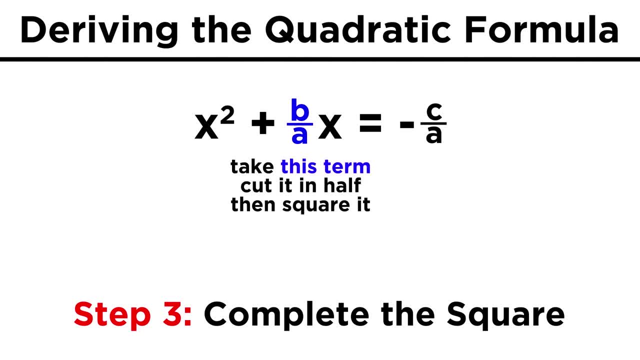 In order to complete the square, we take this term, cut it in half and then square it. It may seem trickier with variables instead of numbers, but it's really the same thing. so we get b over two, a, since dividing by two just puts a, two in the denominator. and 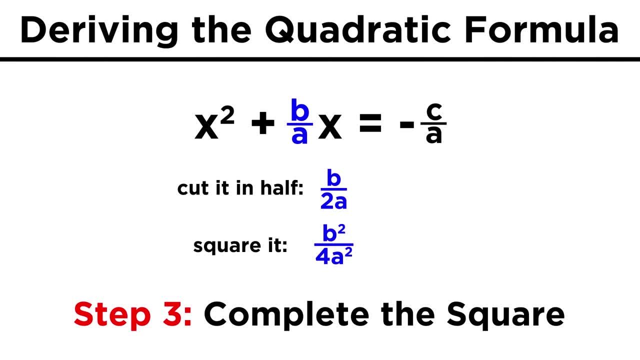 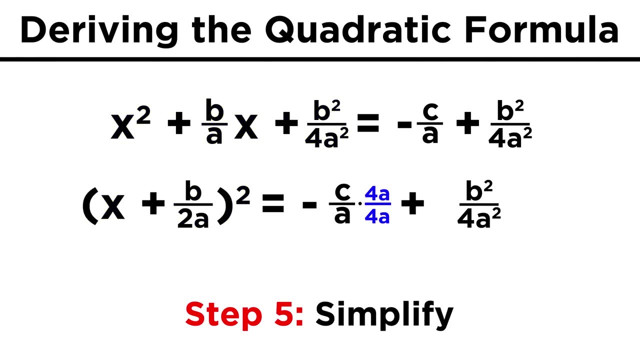 then squaring gives us b squared over four, a squared. This term will be added to both sides. Now, on the left we have a perfect square, So let's factor it and get x plus b over two, a quantity squared, while on the right, 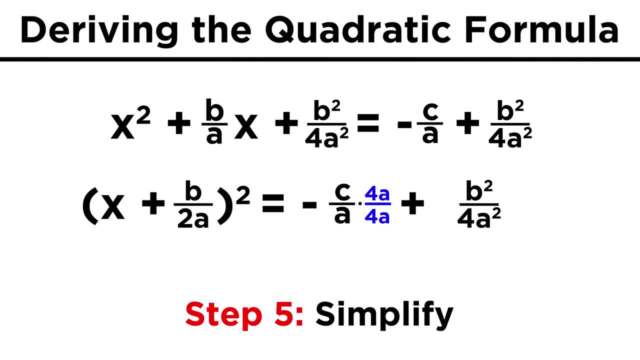 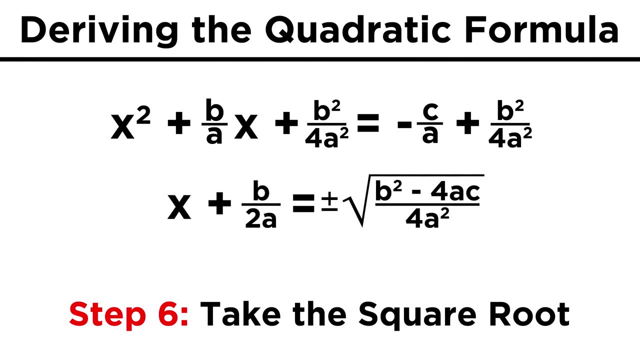 we can multiply c over a by four, a over four a, so that we end up with the same denominator for both fractions, allowing us to combine them into one fraction. Now we can take the square root of both sides. For the left, that just gets rid of the exponent. 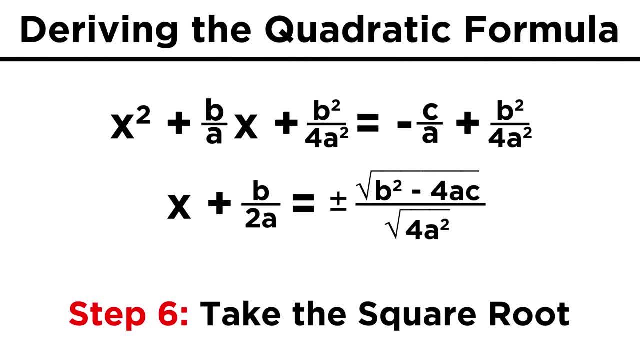 On the right. instead of one big radical, we can put one on the numerator and one on the denominator. The numerator can't be simplified, so let's leave the plus minus there, but the denominator is a perfect square, so we can change that into two. a. 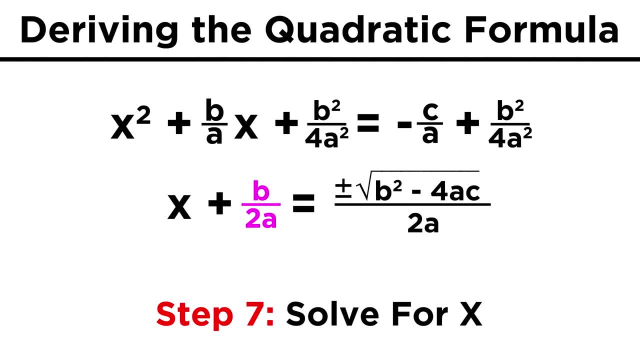 Now we just subtract this term on the left from both sides to get x alone recognize that these have the same denominator. so we combine them and there we have it, the famous quadratic formula. Even though you just learned how to derive this, it is still a good idea to take the 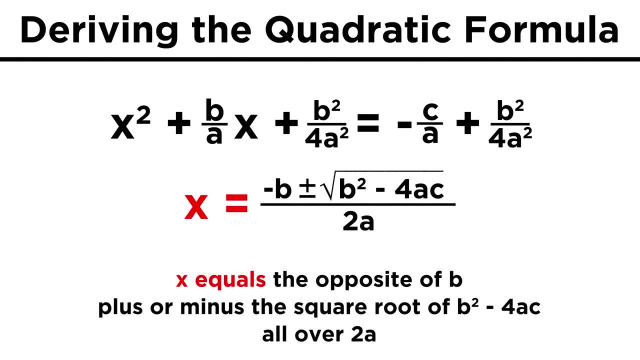 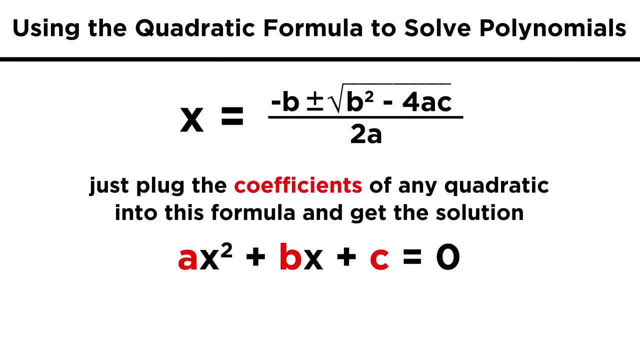 idea to memorize it. so repeat after me: X equals the opposite of b plus or minus the square root of b squared minus four a, c all over two, a. The reason this equation is useful is that we can take any quadratic plug: a, b and. 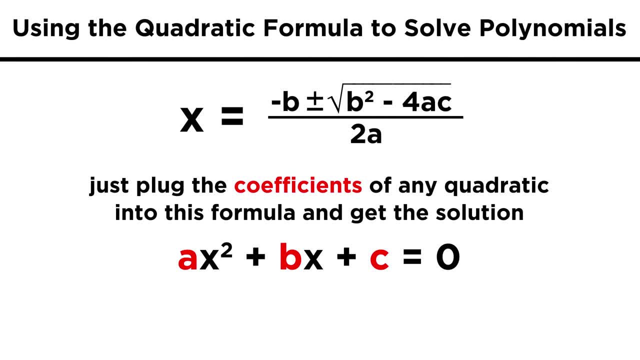 c into this formula and it will spit out the solutions to the equation. Let's try one example now: X squared plus two, x minus three. Now we should be able to see from our knowledge of factoring that this can easily be expressed as x minus one times x plus three, meaning that the solutions are one and negative three. 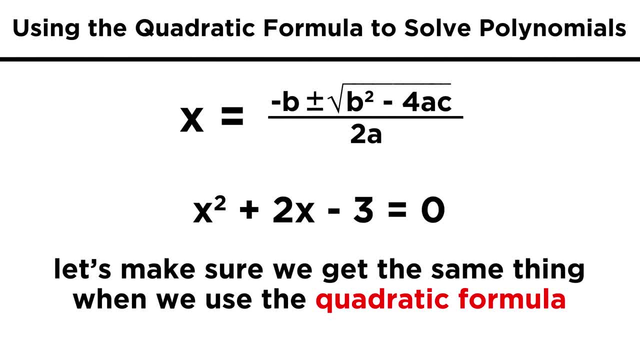 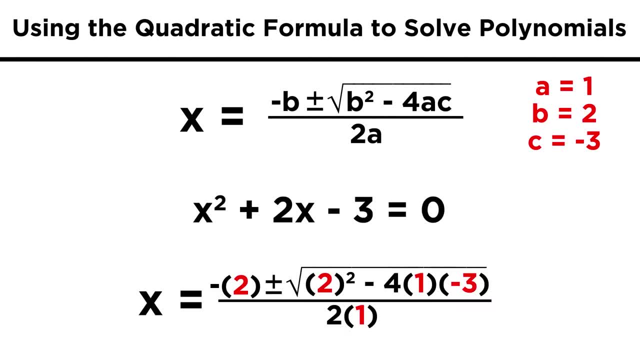 But let's plug the coefficients into the quadratic formula to make sure it works. A is one, b is two and c is negative three. so let's just replace all of these variables with the corresponding numbers. Now we just simplify step by step. 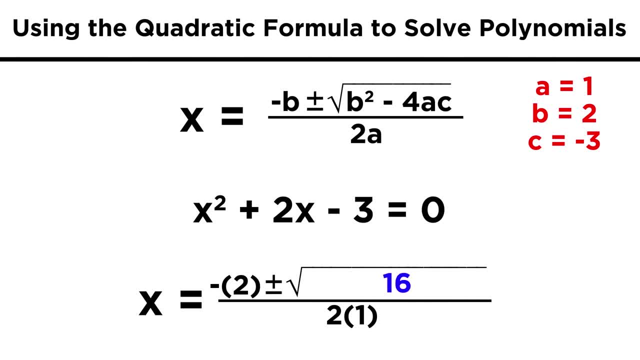 Let's combine everything under the radical to get sixteen. Take the square root, which is four, and now we have two answers: negative two plus four over two or negative two minus four over two. These give us two over two and negative six over two, which is one, and negative three. 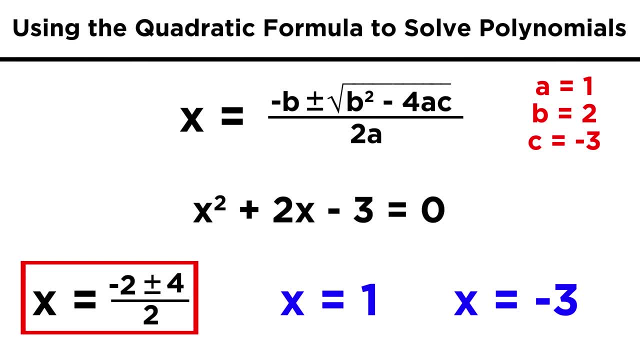 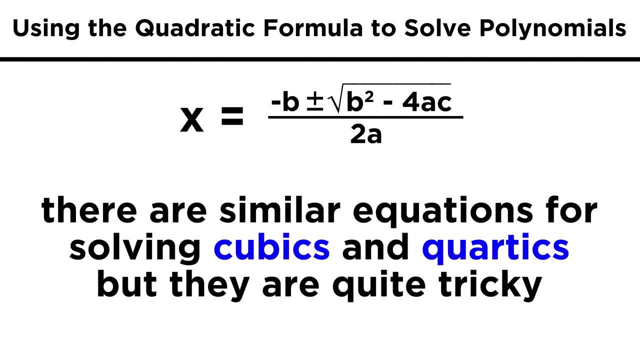 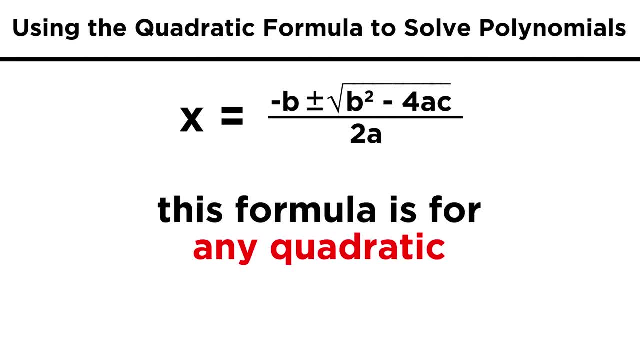